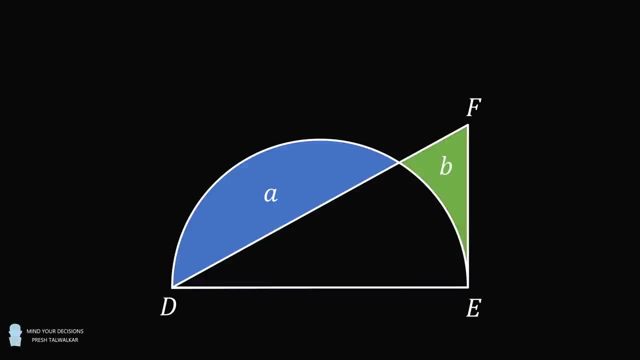 in the triangle have an area equal to B. If A is equal to B plus 47 and DE is equal to 20, what is the length of EF? I thank Min for the suggestion. Pause the video if you'd like to give this problem a try and, when you're ready, keep watching to learn how to solve this problem. 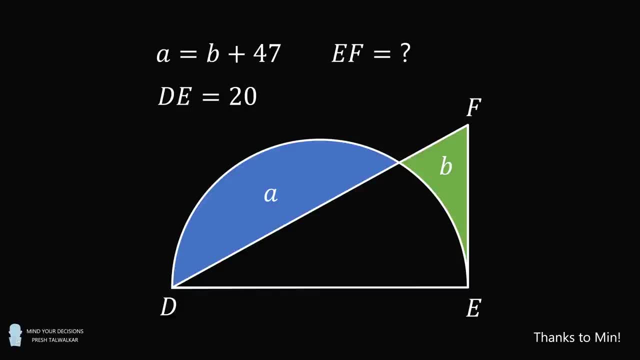 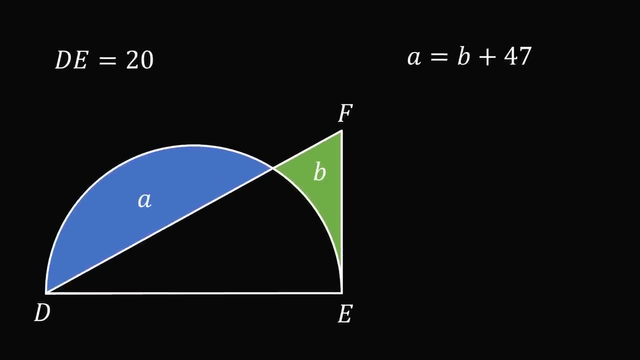 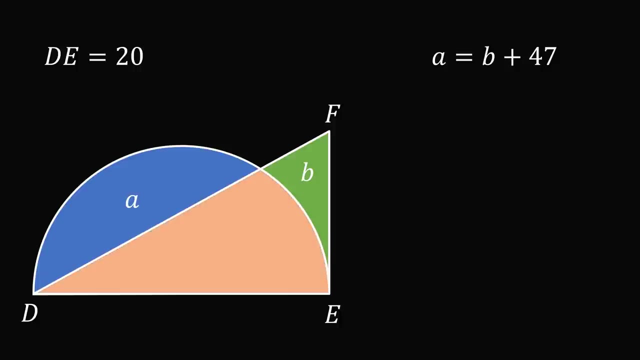 There's a very neat trick to solve this problem. Consider the third region, where the semicircle and the exterior of the semicircle have an area equal to B. Let the region contained in the semicircle right triangle overlap and suppose it has area C To the equation: A is equal to B plus 47,. 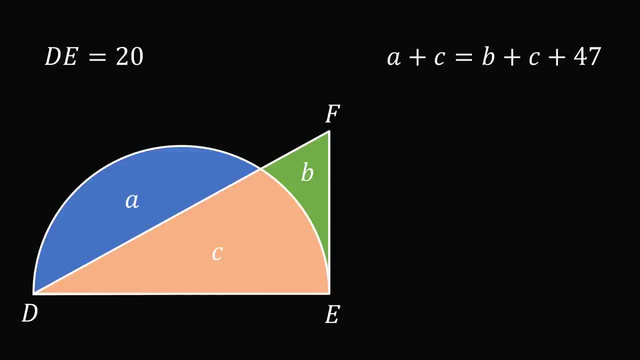 add the area C to both sides, We now have A plus C is equal to B plus C plus 47. But what is A plus C? It's exactly the area of the semicircle. The area of the semicircle is equal to pi r squared over 2.. 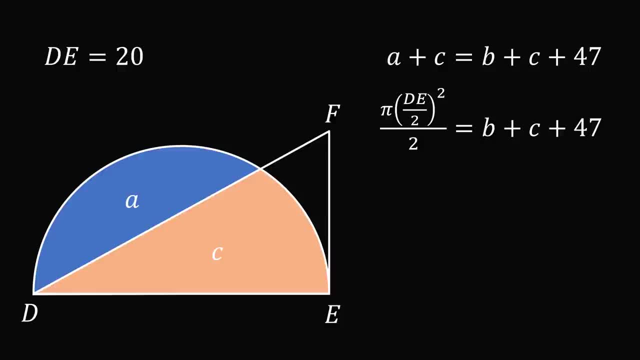 In this case the area of the semicircle is equal to pi r squared over 2.. In this case, r is equal to DE over 2.. This will be equal to 10.. So the area of the semicircle is 10 squared pi, all over 2,. 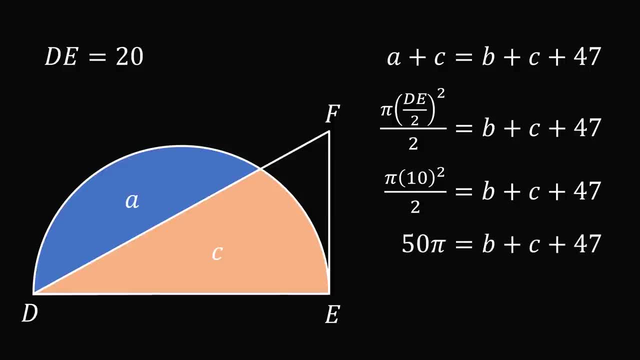 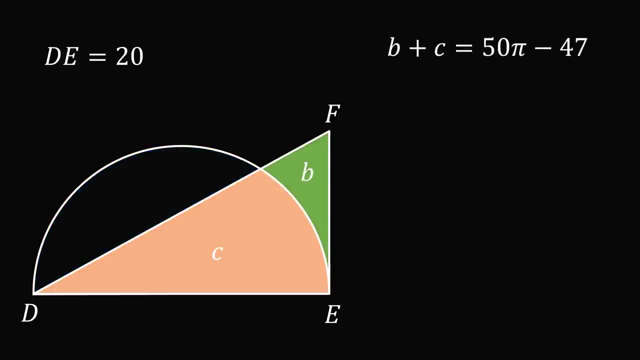 which is equal to 50 pi. We then subtract 47 from both sides to get B plus C is equal to 50 pi minus 47. But what is B plus C equal to? This is exactly the area of the right triangle, DEF, And the area of the right triangle is equal to DE multiplied by EF all over 2.. 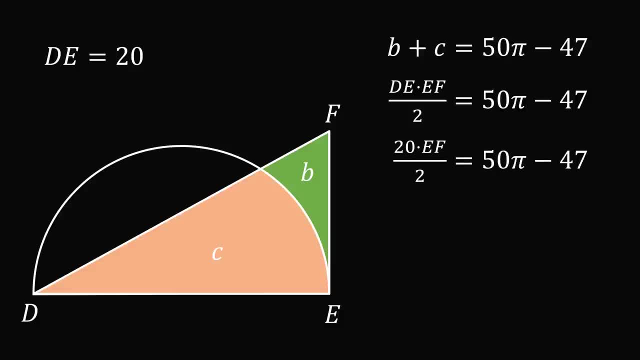 Substituting DE is equal to 20, and then dividing by 2 gives 10EF is equal to 50 pi minus 47.. Dividing both sides of the equation by 10 gives EF is equal to 5 pi minus 4.7,, which is approximately. 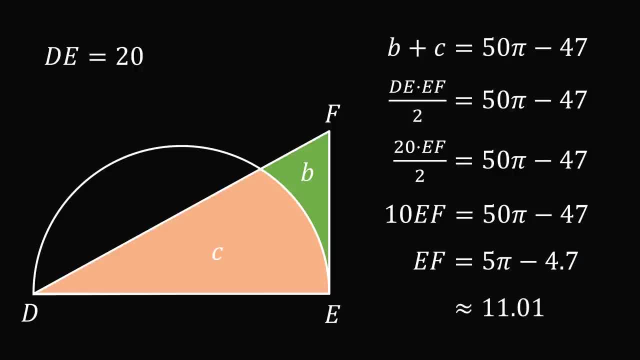 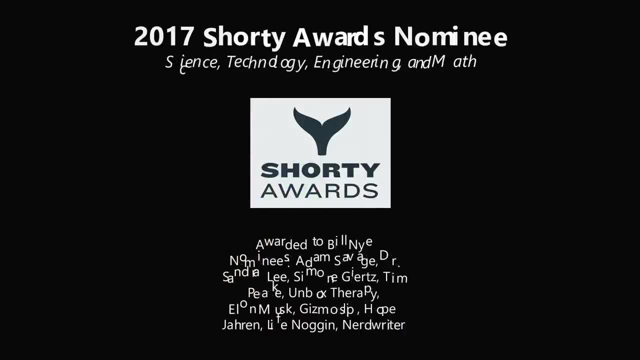 equal to 11.01.. And that's the answer. Thanks for making us one of the best communities on YouTube. See you next episode of Mind Your Decisions, where we solve the world's problems one video at a time.